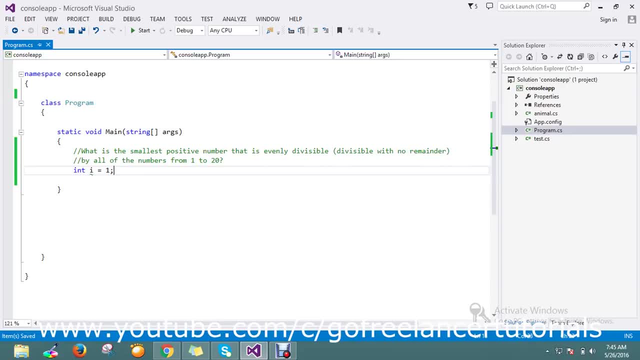 I equal to 1.. Okay, So I just initialized Okay, I want to find out my smallest positive number to divide by 1.. Okay, I just used while loop Okay In while I just go on the just divided condition. 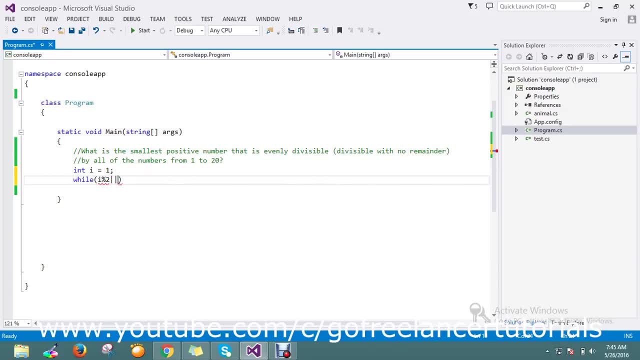 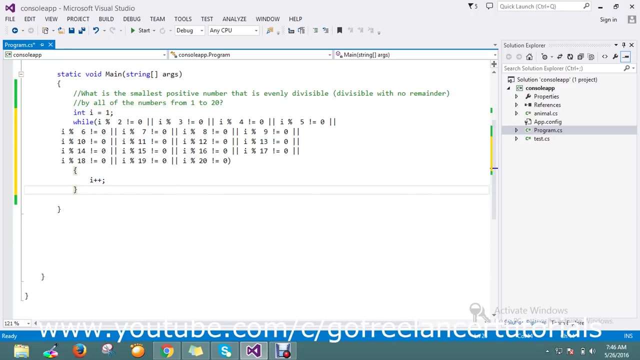 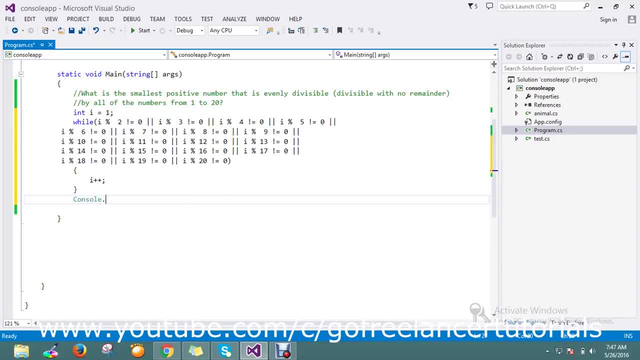 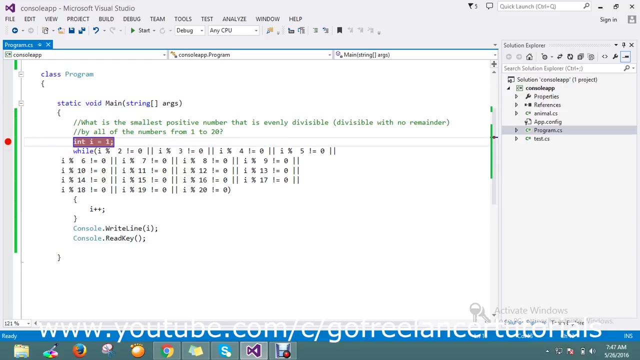 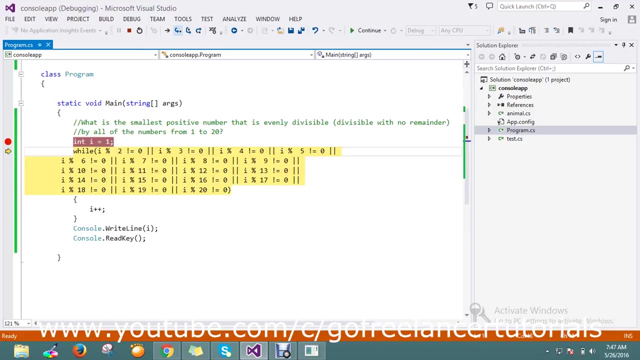 I just to go on right console dot write, line I, and finally I just took console dot read key. okay, good, so let me keep the breakpoint for some times because it will be lengthy process. okay, so how this is work like it's check the condition, okay, but it's failed actually. 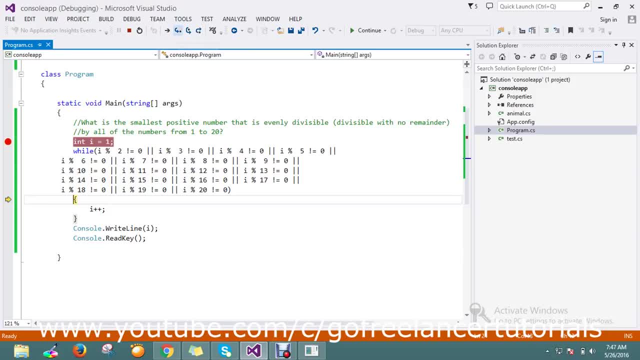 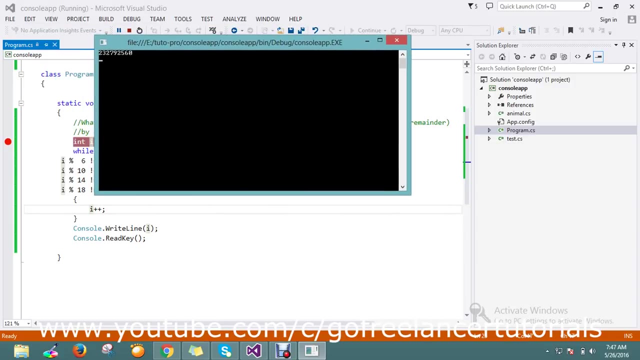 because it has the remainder. so it's gone. incremented my variable like this, it's get looped, so I just keep the continue. so it's took me something around the earlier one second to get the result. yeah, this is the first number, a smallest number and not